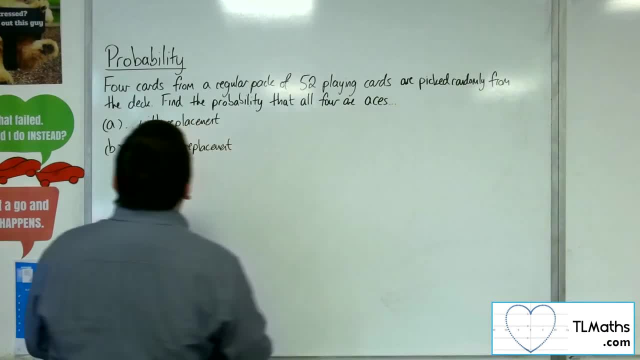 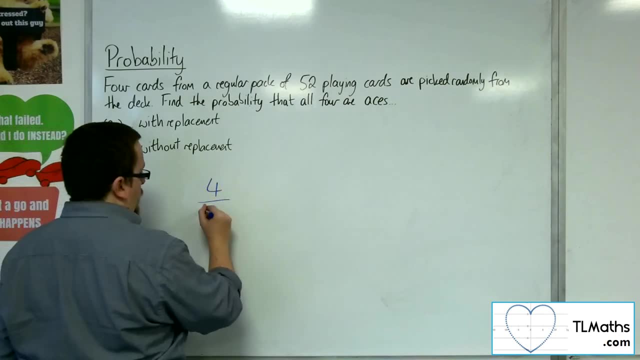 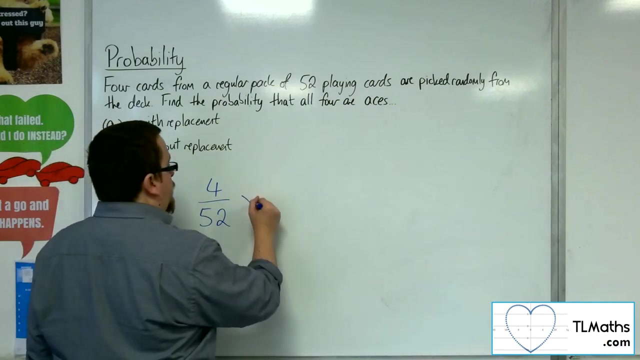 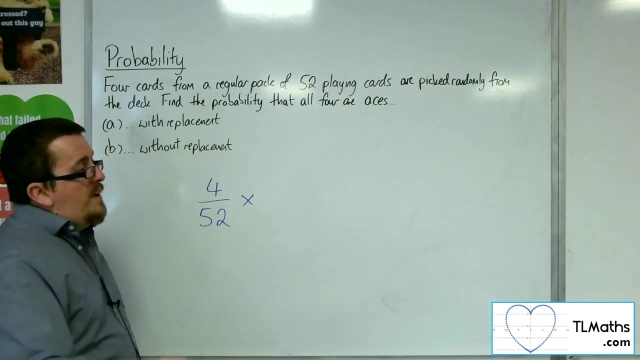 Okay, so the probability of picking out the first ace will be four. Okay, so the probability of picking out the first ace will be four out of the 52.. Okay, that will be the first possibility Then, okay, we've then got, if I replace the card, well, now I've still got four aces to pick out out of the 52 cards. 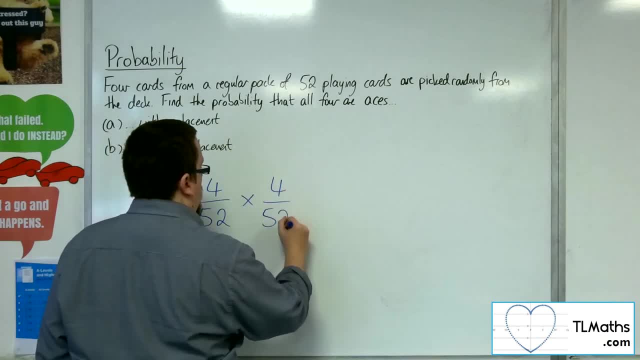 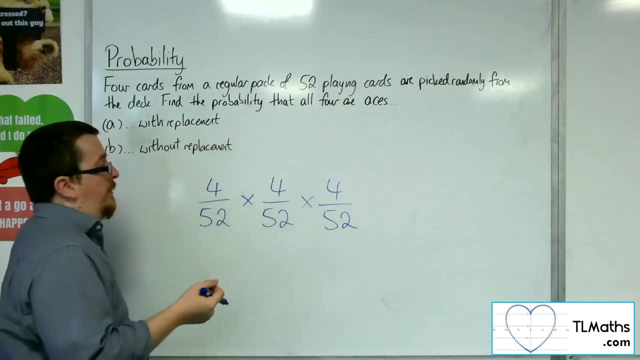 Okay, so I've replaced the card. Okay, so I've replaced the card. I've then got four out of 52 again. for my third choice: I've replaced the card, So I've now got four out of 52 again. 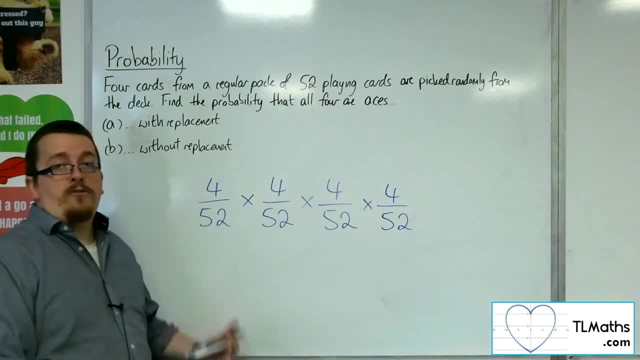 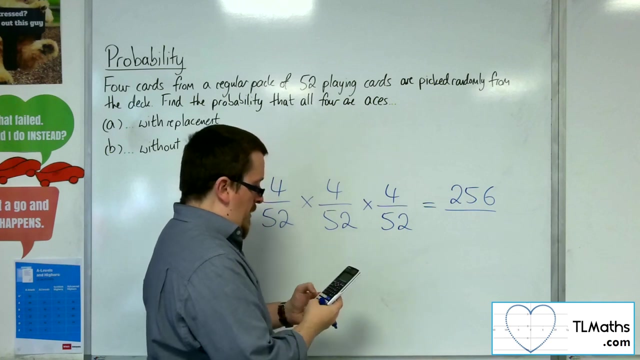 Okay, so this is just four over 52 to the power of four. Okay, so four to the power of four is 256.. And 52 to the power of four is 75.. 73, 1, 1, 6, 1, 6.. 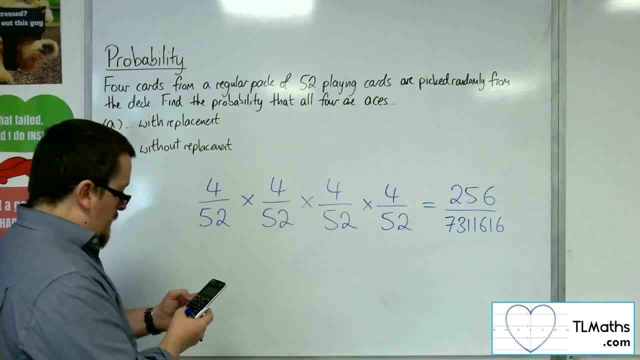 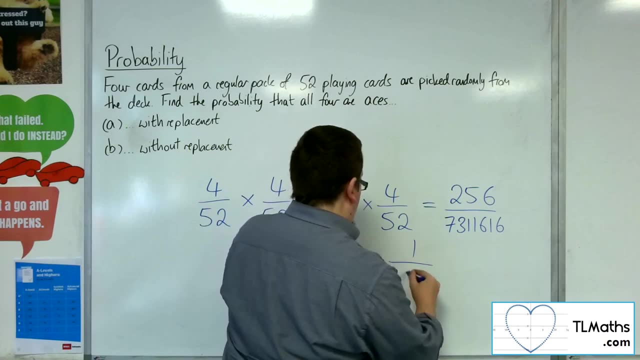 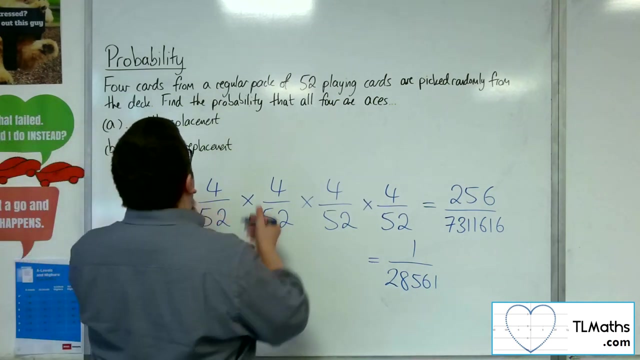 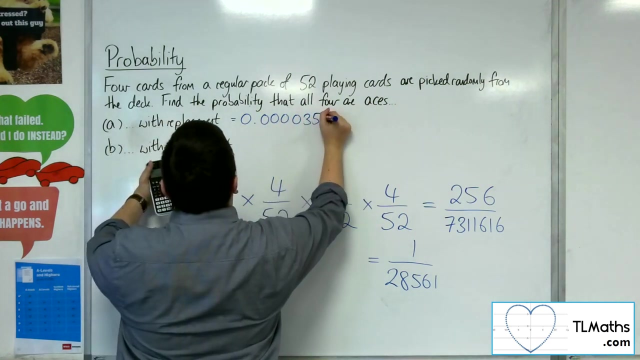 So we want that to the power of four, don't we? Okay, so this simplifies to 1 over 28,561.. Okay so, that is 0.00000350.. Okay so, this simplifies to 1 over 28,561.. 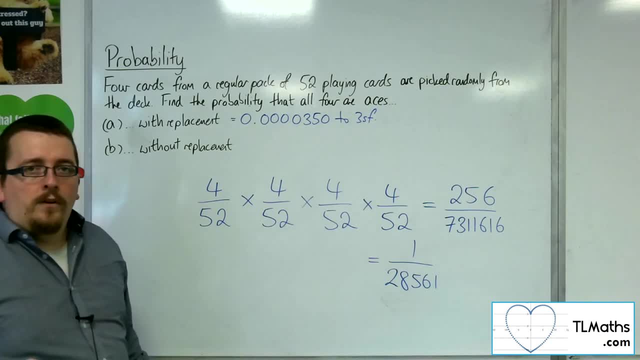 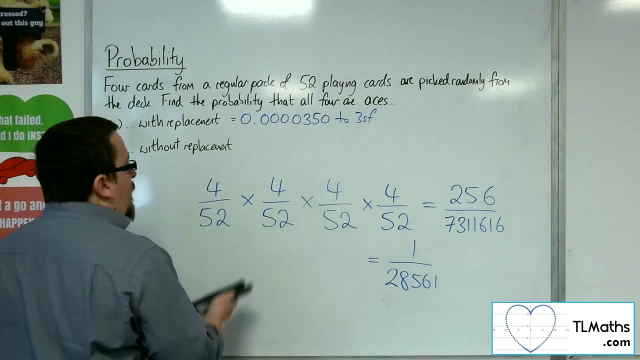 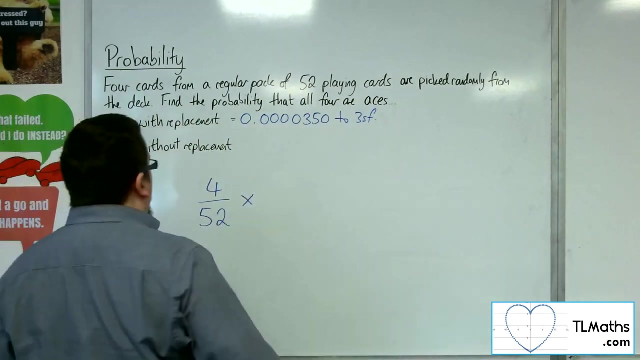 Okay, so this simplifies to 1 over 28,561.. That's the probability of picking out all four aces if I replace the card. Okay, right, So if I now don't replace the card and I remove it each time, the first pick will still be four out of 52.. 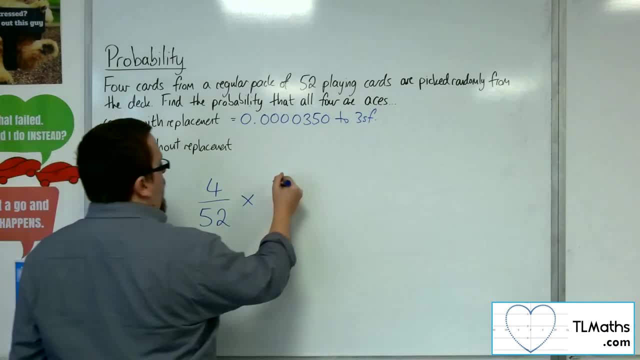 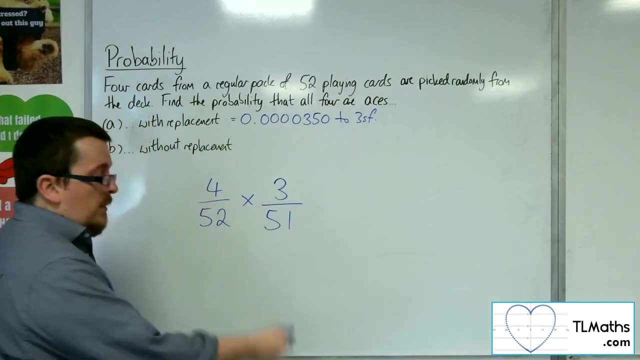 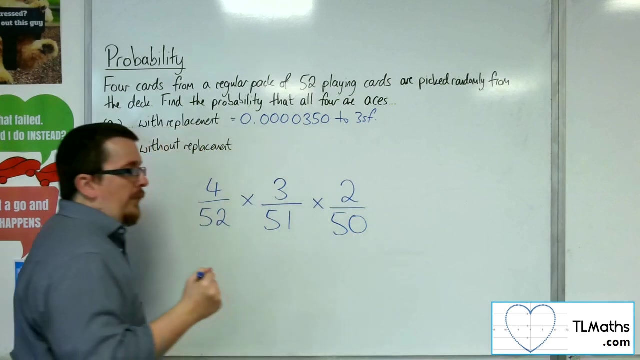 But now that I've removed that ace, there will now be three aces left. There will now be three aces left out of 51 cards. I pick that ace out, I remove it, So I've now got two out of 50 cards left.